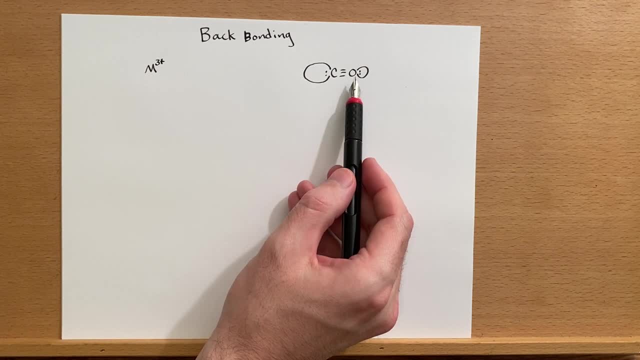 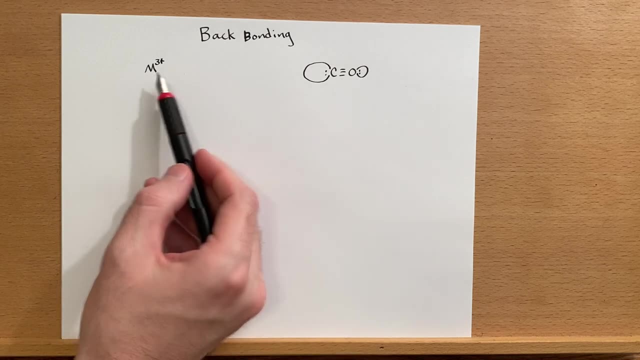 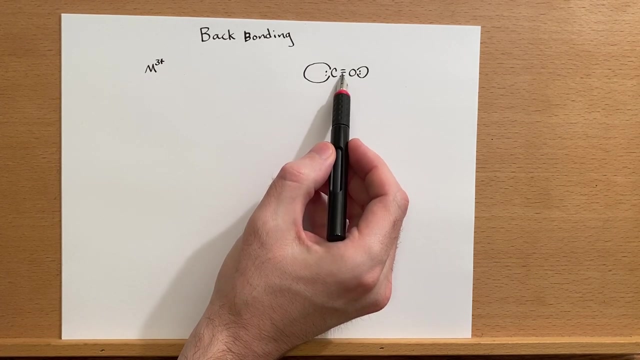 is the negative side of this molecule, that one's electronegative, This side's negative. This thing is positive. We would expect that the oxygen would bond to the metal. Well, it just so happens that carbon over here has kind of it has an octet right, but it has. 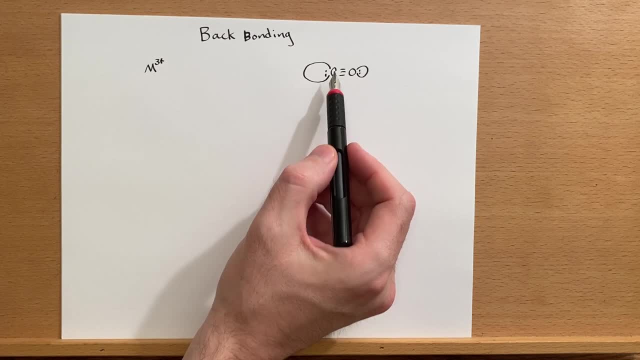 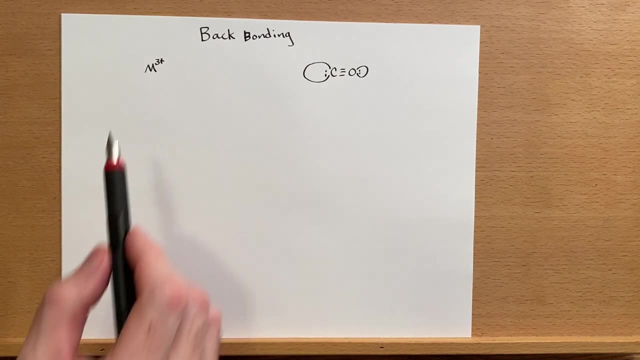 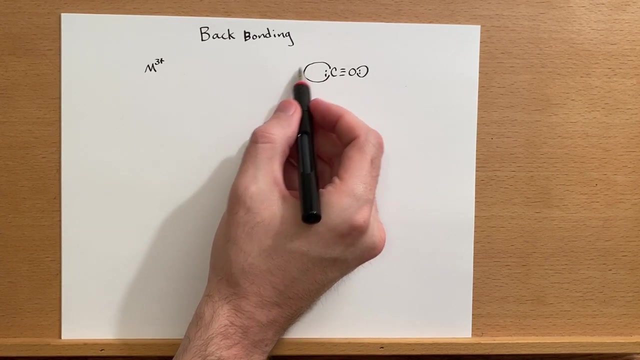 a little bit more electrons around it than it might like, and so it's just a little easier for this to give away electrons, And again the size of the orbital matches up a little bit better with the metal. So in the first case, this sigma orbital right here is going to give its electrons. 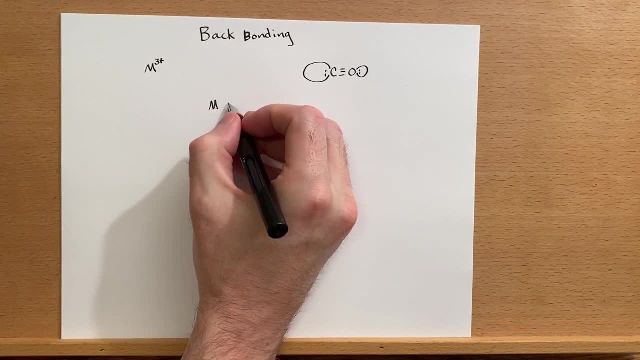 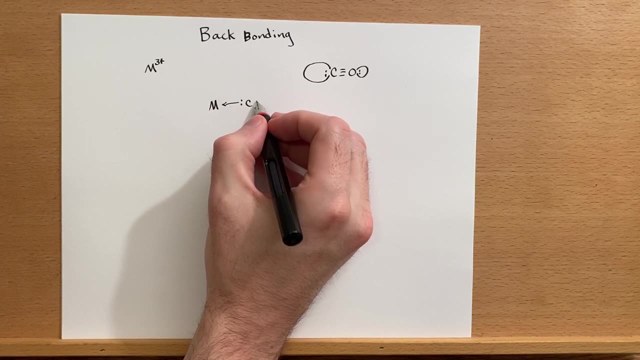 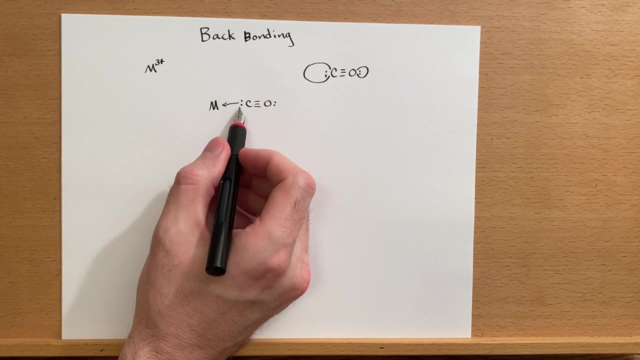 to the metal and I'll draw that right here And I'm going to use an arrow to indicate that both electrons are being donated to the metal Now. this is a very strong donation and it's going to push up the EG orbital to a higher. energy level, and that will cause a higher field or eventually lead to lower spin, because the orbitals are further apart, and then there's less chance of the electrons being paired or unpaired. Now, that's not all of the story, and that's. 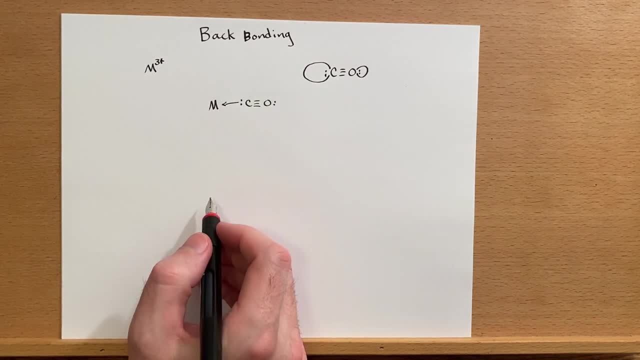 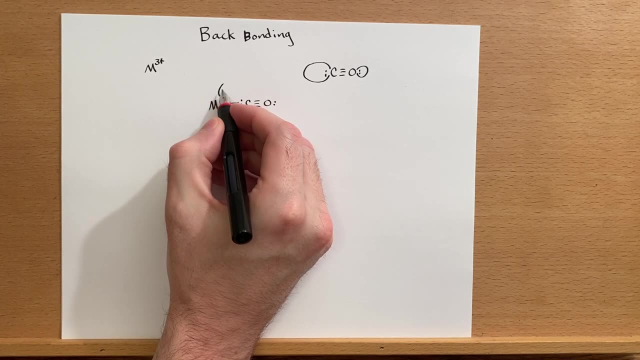 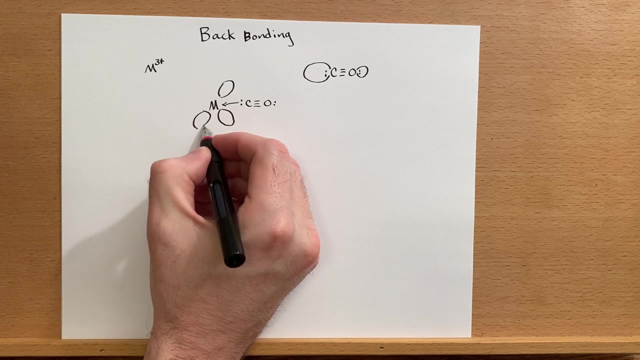 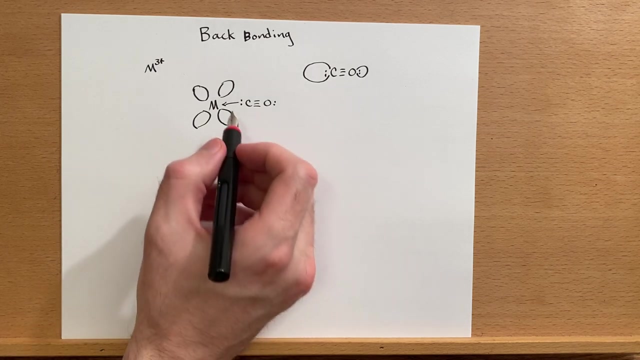 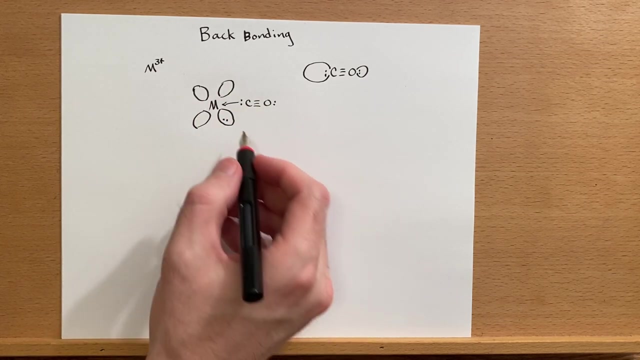 not at all explaining the title of this video: Backbonding. Well, the metal has orbitals of its own like this. Here's one of the d orbitals and that will have electron density in it. You know there's some electrons in here. Well, maybe they're not both in the same orbital. 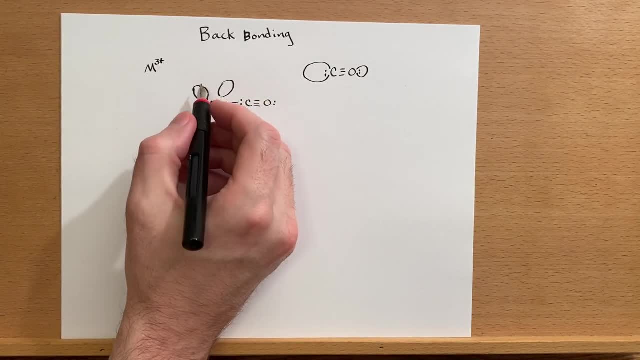 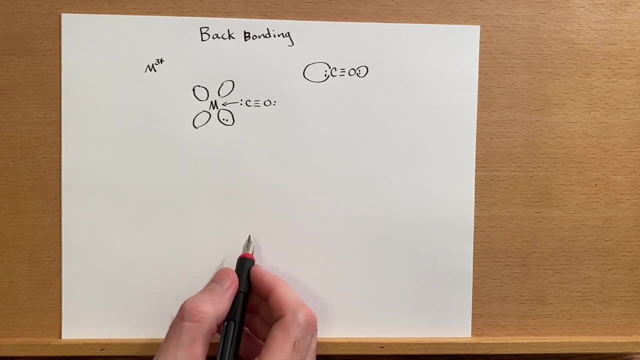 Some might be up there too. In any case, remember there's metal orbitals, and they do look like this. Now, one thing that we didn't focus as much on when we drew Lewis structures and drew the pi orbitals might be the shape of the antibonding orbital. 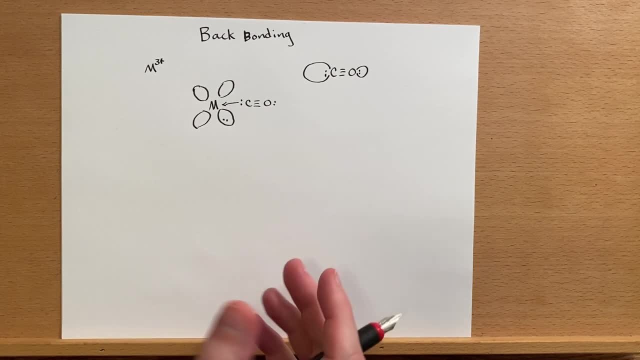 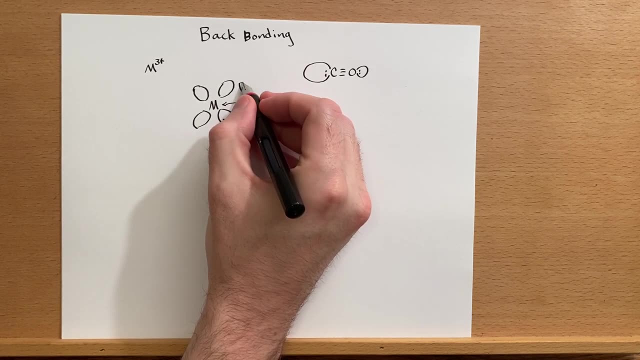 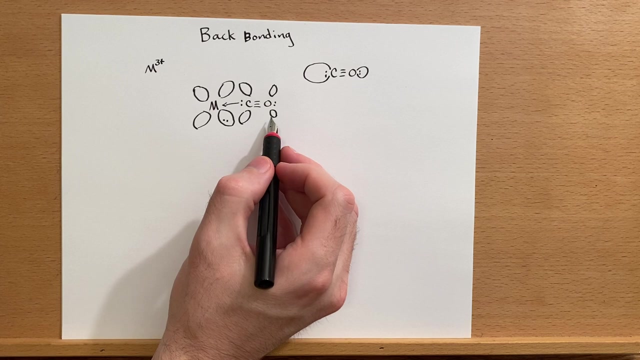 Now, if you look at this, you can see that there are two d orbitals on the carbon monoxide, So I'm going to draw that for you. I'm trying to draw the oxygen orbitals a little smaller than the carbon ones, simply because that's. 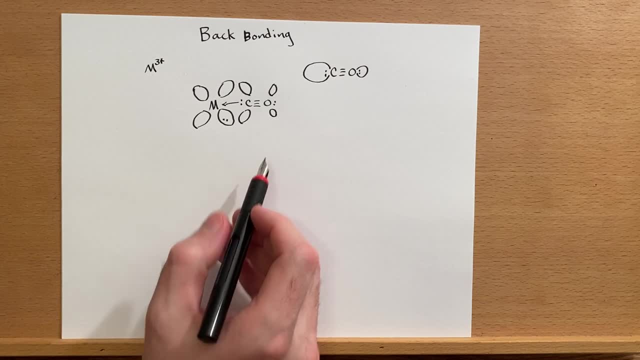 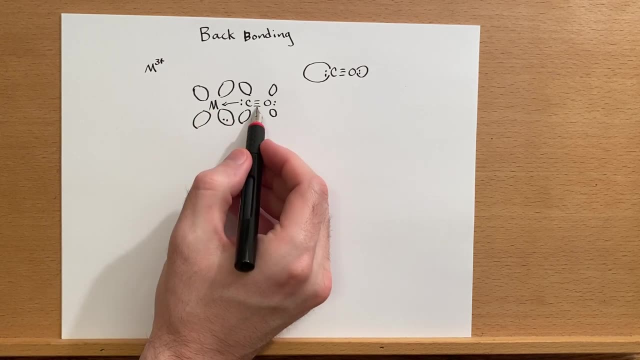 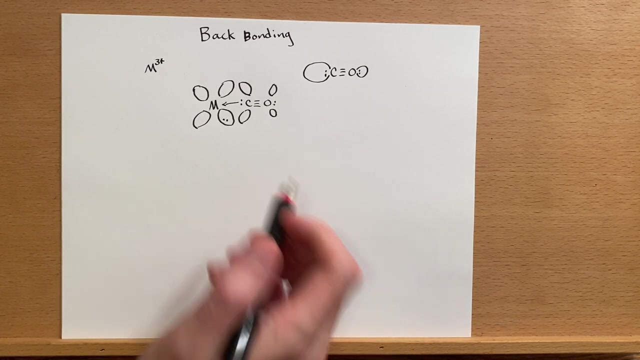 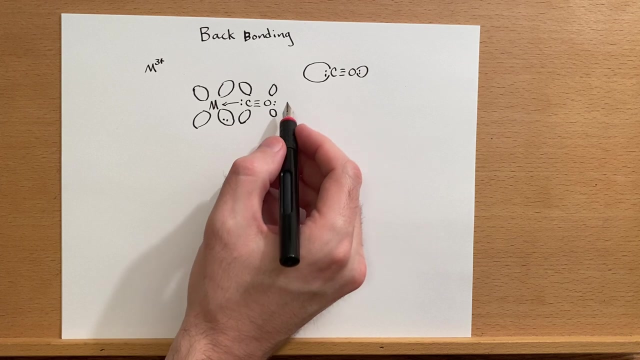 the truth. Oxygen holds its electrons a little tighter. Now this orbital is empty. but when we have the metal bonding with carbon monoxide, electrons like to spread out as much as they can and these electrons here notice that there's an empty orbital, the pi antibonding orbital. Now these are antibonding, because this is a different. 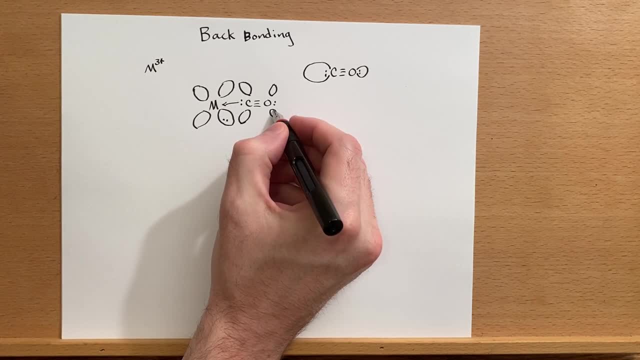 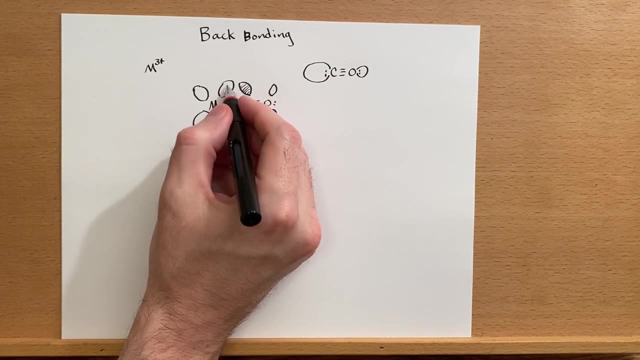 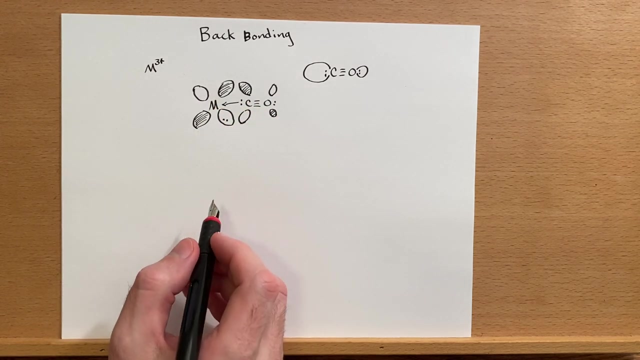 phase. So, if you recall, we would shade in some orbital here and we would have a little bit less of a and we'd shade in that orbital there. Well, these are also phased and we could have kind of like that kind of picture. Well, you can notice that the phase of 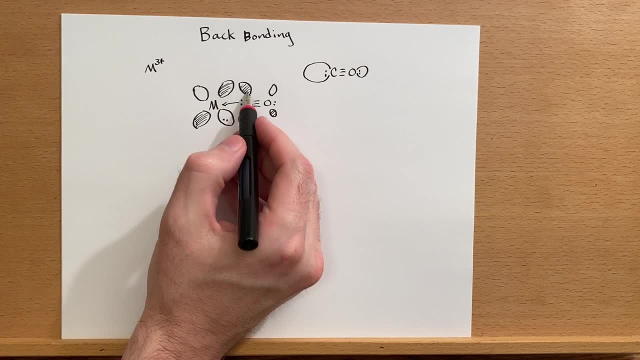 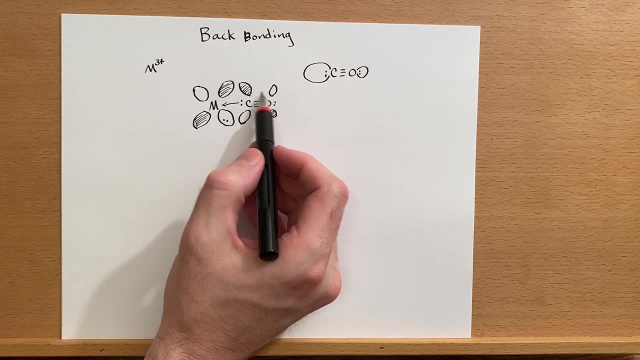 these two orbitals matches up and the phase of those match up so they can interact with each other. and this is why it's antibonding over here, because the phase does not match in between these two. In the bonding orbital these do match in phase and so there is an interaction between these two, but in the 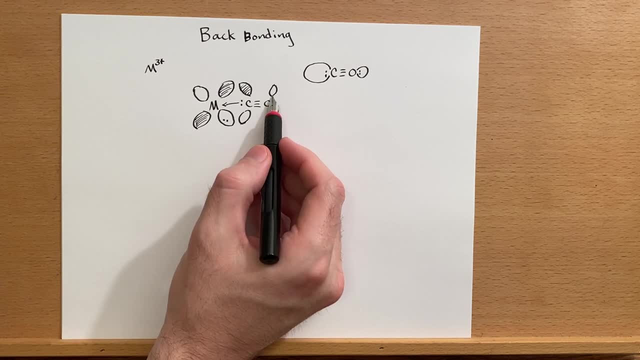 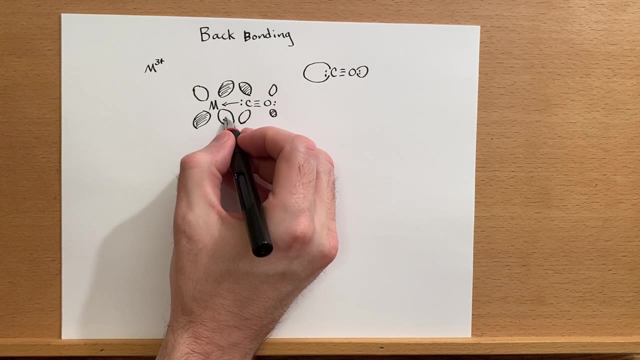 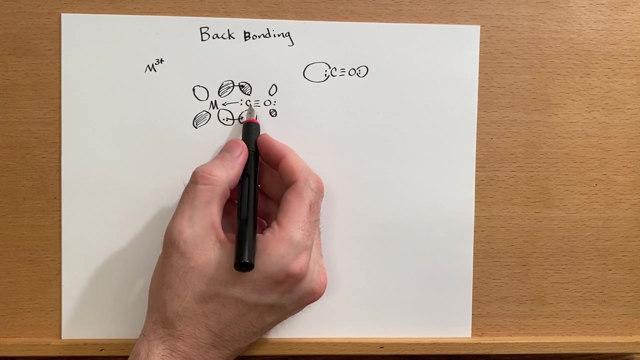 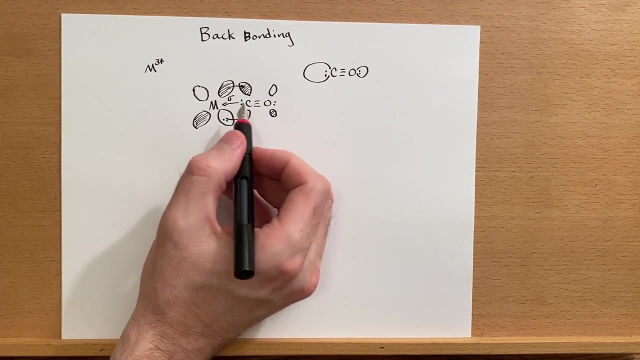 antibonding. these are opposite phases of each other and they combine in a destructive manner. Well, what happens here is these electrons can donate back into this antibonding orbital because we have some Sigma donation coming in. we have some Pi back bonding here. so Sigma is direct overlap and pi bounding is a side-to-side interaction. 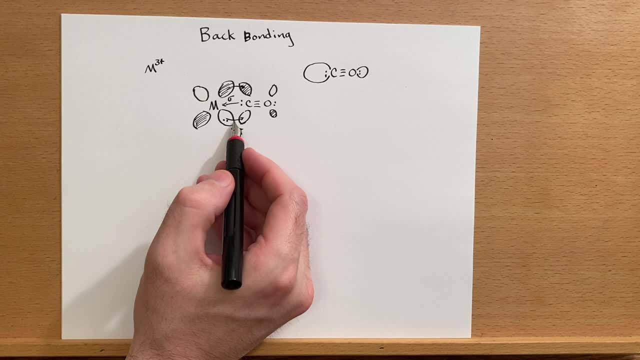 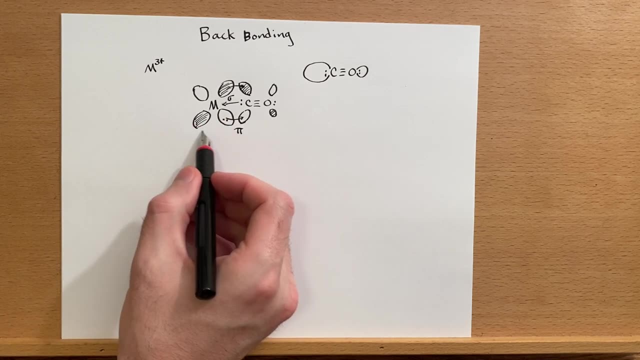 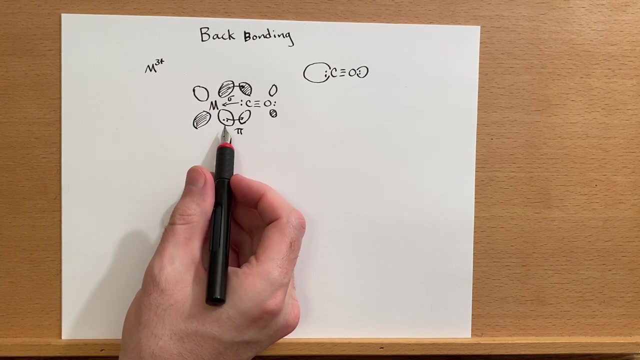 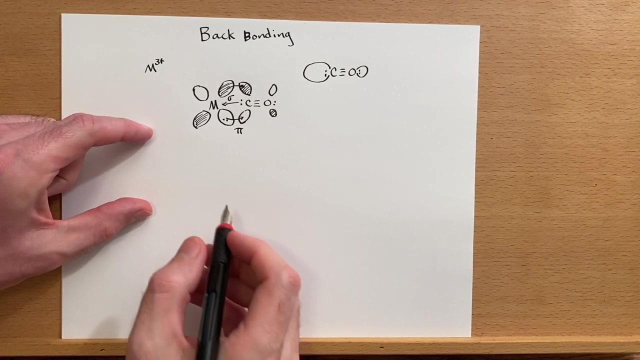 in two locations. Now, what this does is it lowers the energy of these orbitals. Now, this does lower the energy of these orbitals because these are not bound together, But let me just show you a sample: orbitals on the metal. These orbitals are the T2G orbitals. so what that does is, instead of the EG, 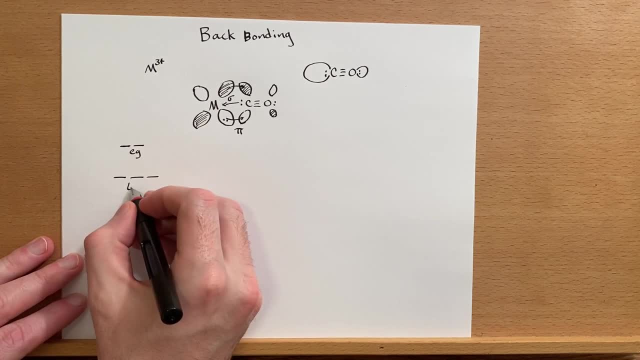 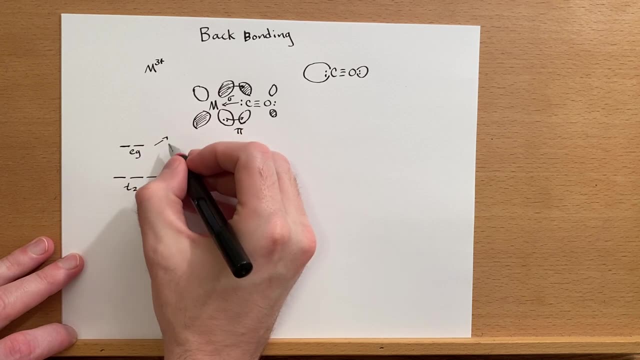 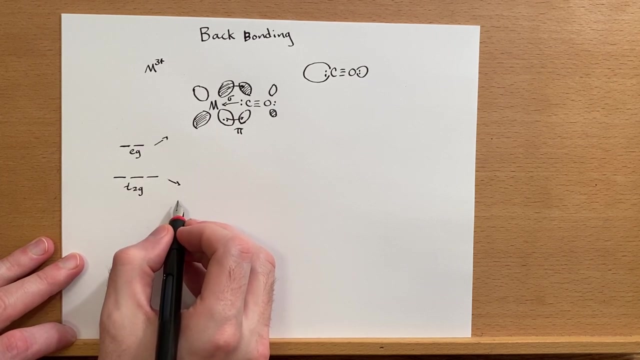 being like this and the T2G being like this: if we have very strong sigma donation, that will push up the T2G orbital and if we have pi backbonding, that will stabilize the the T2G orbital. so it pushes up the EG. 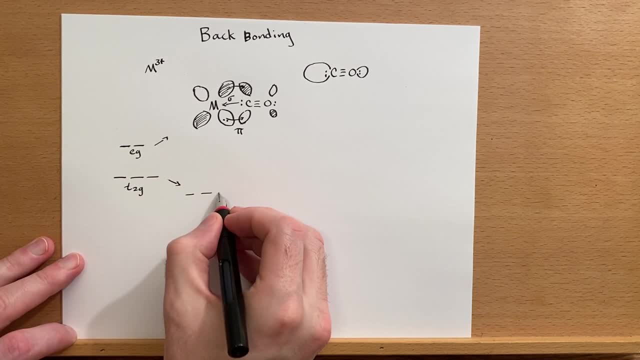 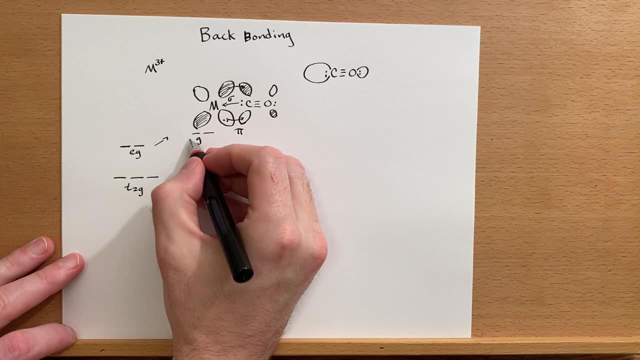 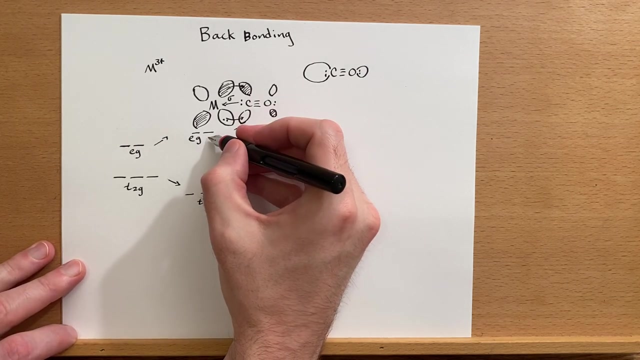 stabilizes the T2G, and the net effect of that is these have an increase in energy density. so that's the difference between them, and since we're in an octahedral environment, we call that the delta octahedral energy. 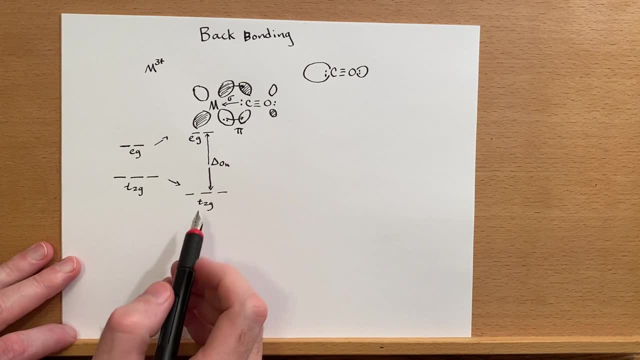 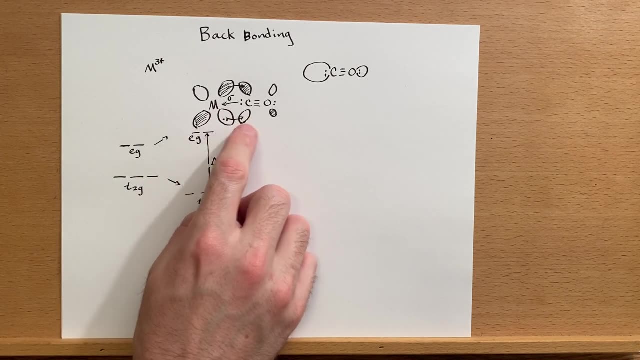 Right there, and that's how backbonding works. Now you might say, hmm, that's interesting, but since this is going into the anti-bonding orbital of the carbon molecule, it's not going to be able to backbond the T2G orbital. so it's not going to be able to. 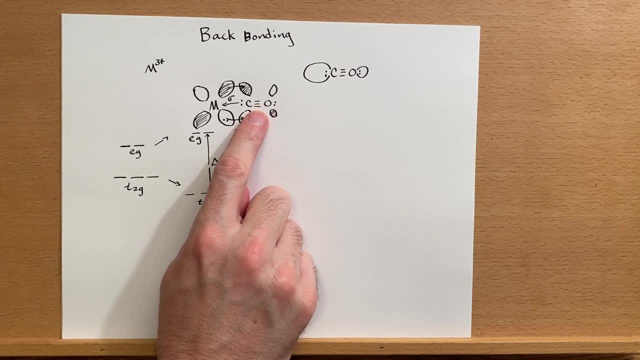 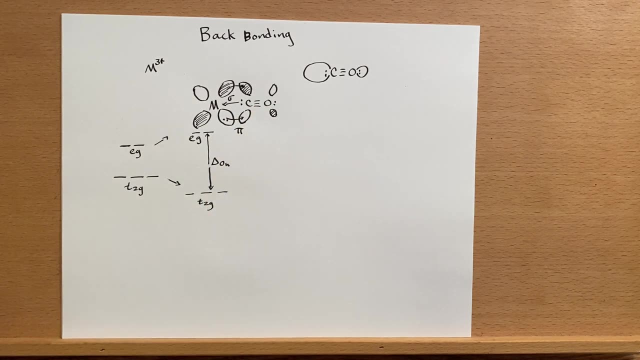 backbond the T2G orbital. so it's not going to be able to backbond the T2G orbital And that's true. It will weaken the bond of the carbon monoxide, and that's one of the things that we can measure. You can use the infrared stretching frequency of the carbon oxygen bond to determine. 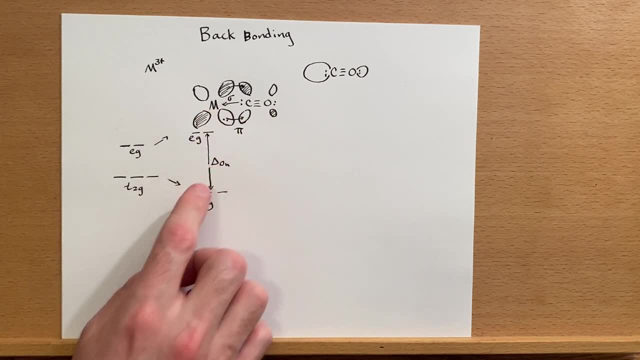 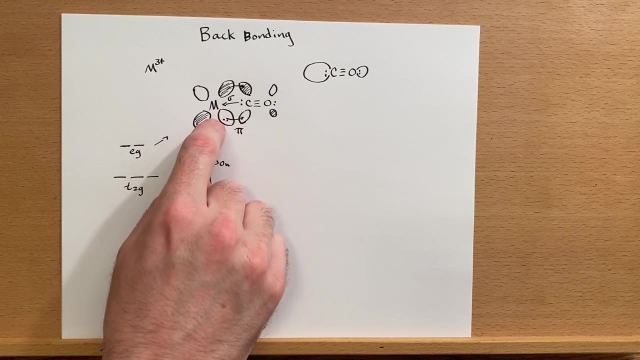 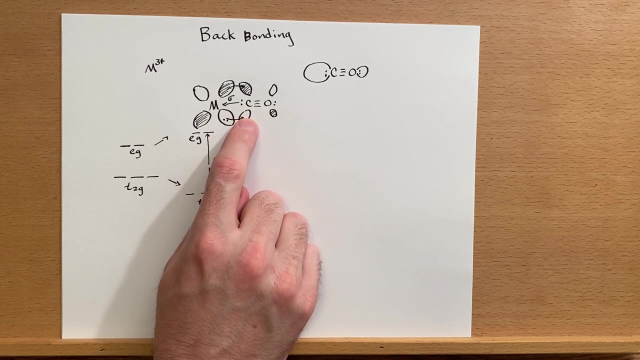 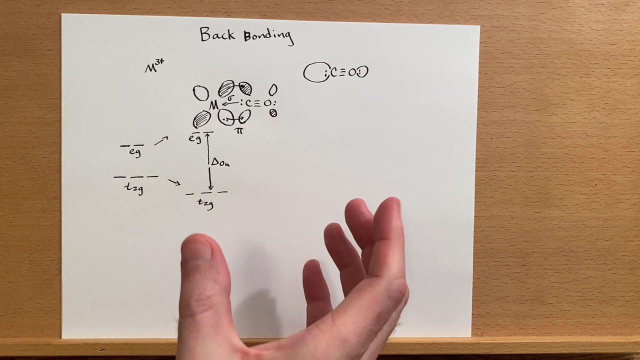 what the electronic character is on the metal. So if the metal is, say, oxidized, then it will have less electrons on it and less donation back to this orbital, and so then this bond will be stronger and the frequency will be higher, because stronger springs vibrate quicker. 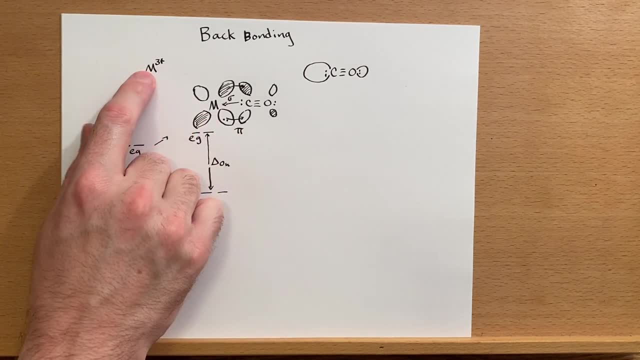 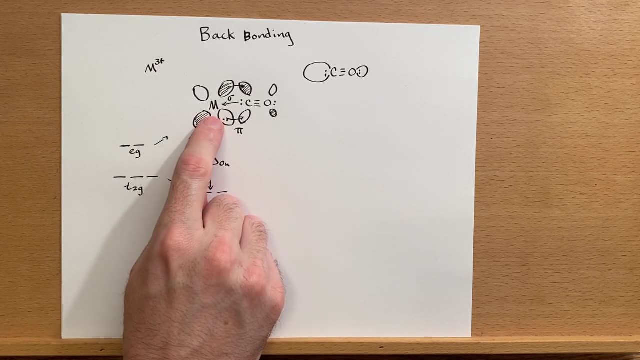 Now, conversely, if instead of this metal being a 3 plus charge, it was say a 2 plus charge, that means there's more electrons on the metal and it has another electron in one of these d orbitals. 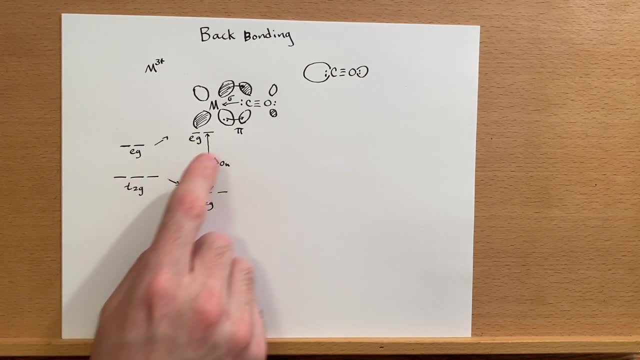 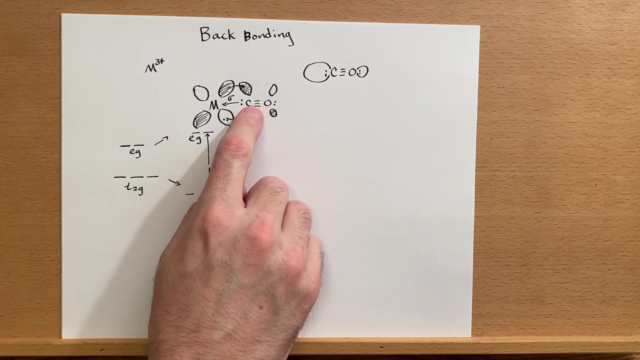 and again, since these are the T2G orbitals that are going to interact with the pi system here, there will be electrons in there, So we'll have more electrons being donated back to the carbon monoxide. That will weaken this bond more and the stretching frequency will slow down.